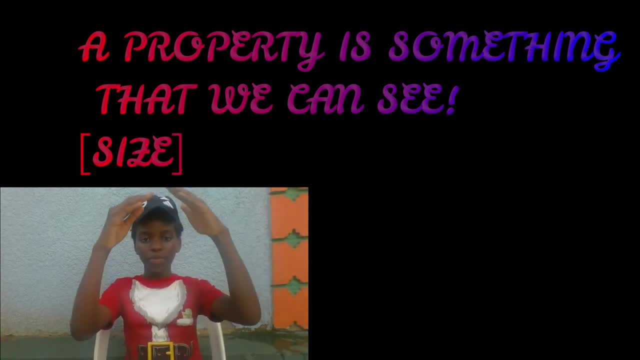 the property of a triangle. A triangle maybe need to be a triangle, need to have, maybe like oblique lines, and I say two oblique lines and one oblique line, So a triangle need to be in one horizontal line. That's a property, yes, And it need to maybe what? 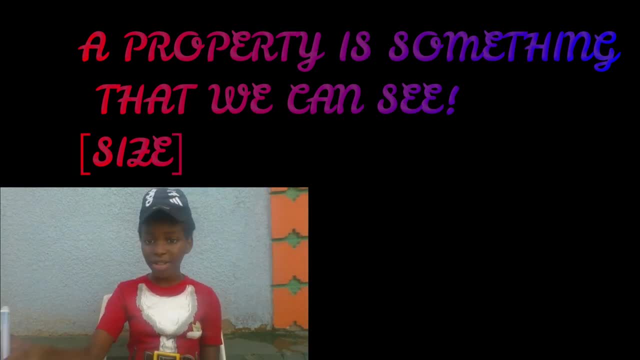 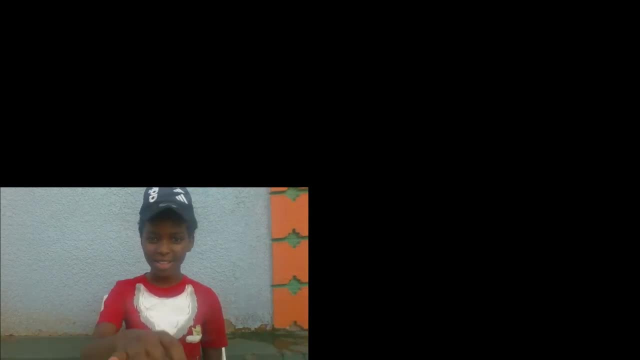 the variety of in the right angle. it need to have 90 degrees, So it's something that you can see when you draw a right angle right. So that is a property. Now we can go. What are solids, Liquid and gas? 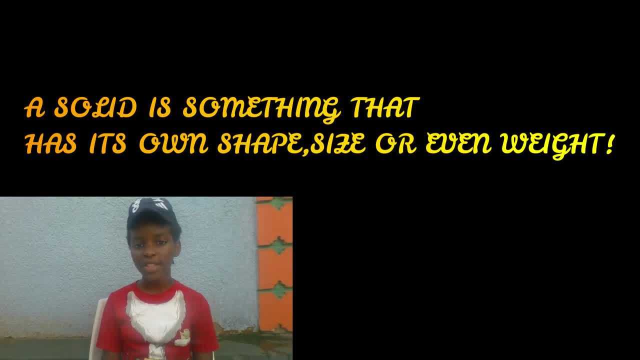 What is a solid? So a solid is something that has it own size. How Let's get an example with this pen: Cada parалась de cada surera está un dígito de drops, pero cada朋友 muestra una suelta. 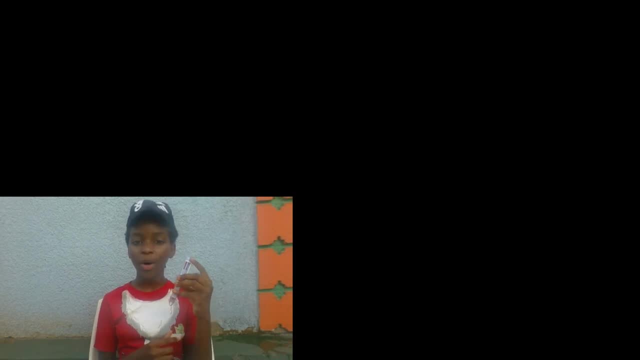 a solid because? why? because it has it called its own size. now, another thing that can define also a solid is: a solid doesn't change size. if you take this pen, you put it here. it can change size. if you take this perfume, you put it here, it. 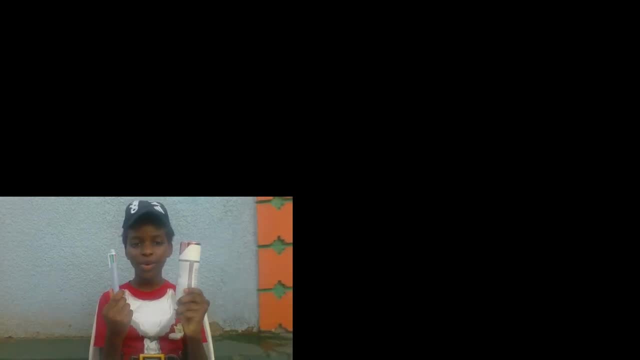 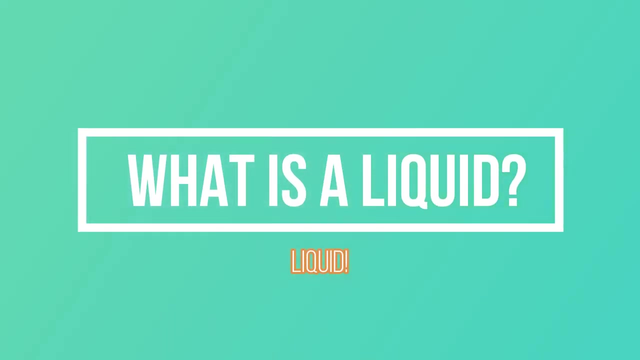 doesn't change size, which means these are solids. why, if they have its own shape, it has its own shape. it is shape when you broke it, so yeah, it breaks. it cannot again come back to normal, to its original form, so yes, it has its own size and it can change when you replace it. now let's go to what are liquids. 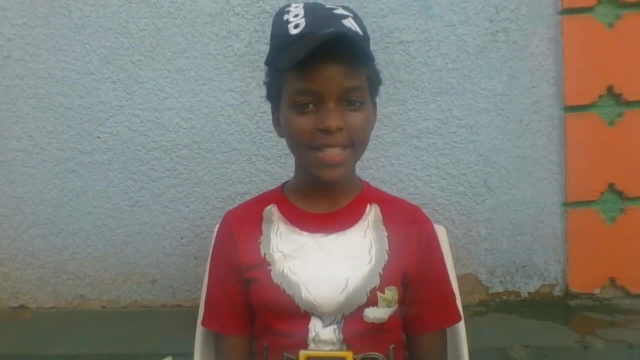 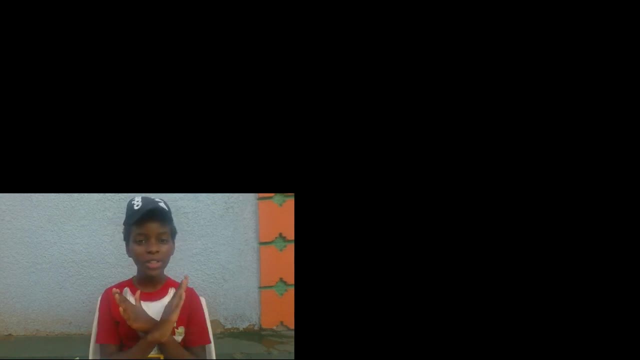 okay, guys. now what's our liquids? so liquids are actual things that take the size of each container, so it doesn't have its own shape like a solid and it has only it's the amount you can get, amon, but just the only difference is that it. 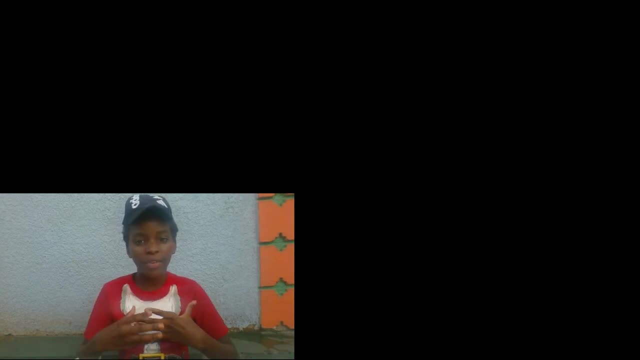 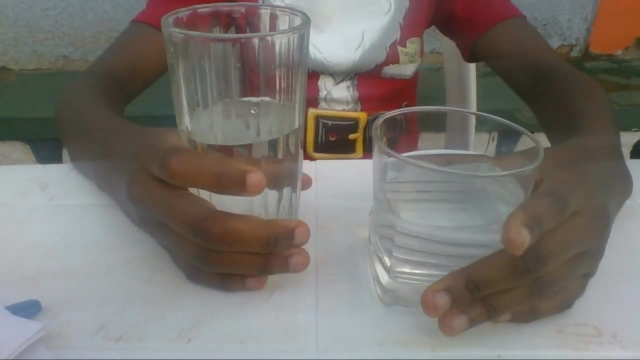 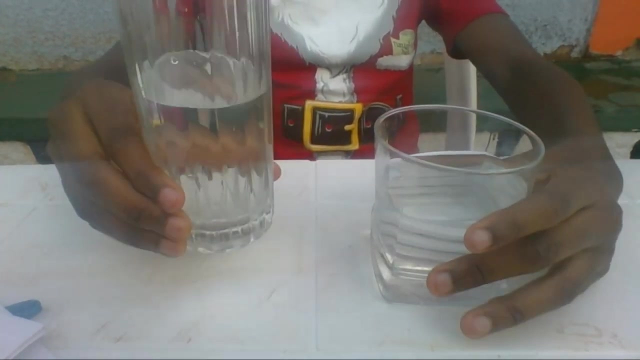 take the size, or you can you take the shape of it container, for example. look at these two verses: full of water, less instead, really well, so, here, dear, as I said, it did take the shape of its container. you see, this container, this glass and this one are 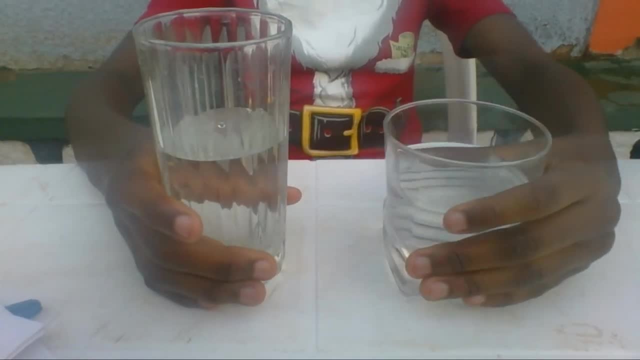 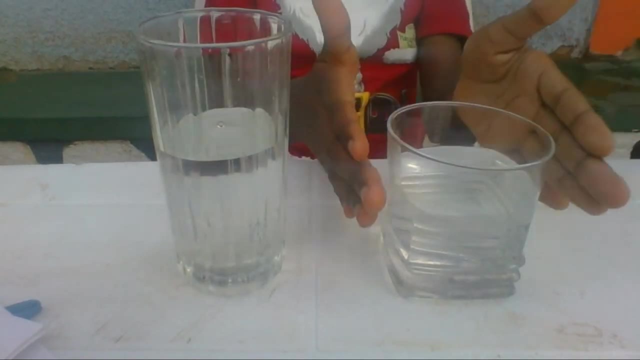 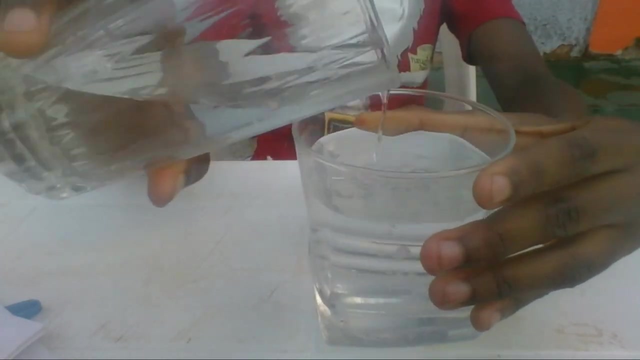 totally different, but, as you can see, it take the size of only its container. this one is actually going vertically. this one it's a little bit large. so see, they have different shapes. when i put in, it keeps going like this, but then it just have the shape of its container. that's what you call a. 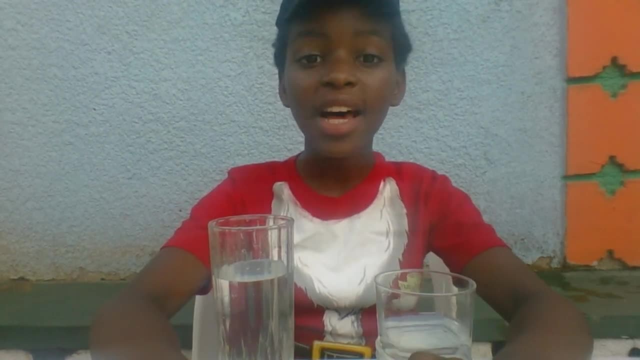 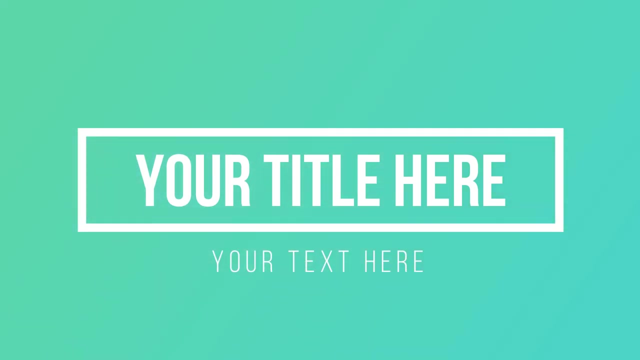 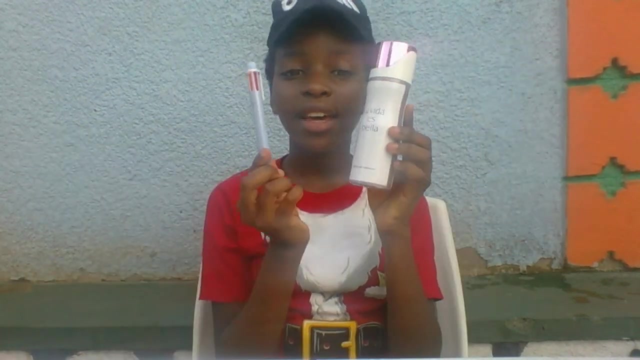 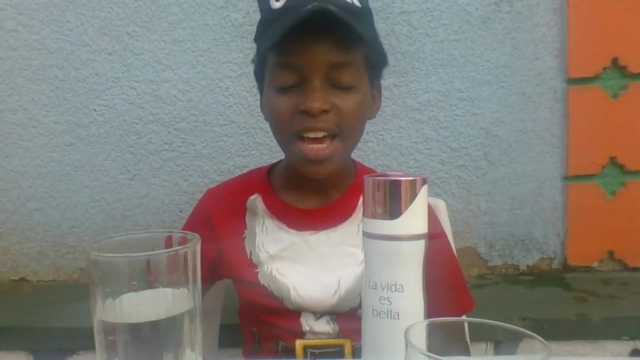 liquid. that was actually easy. now let's go to words. are actually: what is the gas? okay, guys, i guess it actually is very different from audio, from saying it's needed, so it you cannot see it. but it's totally different how it, because the guys you cannot see them. 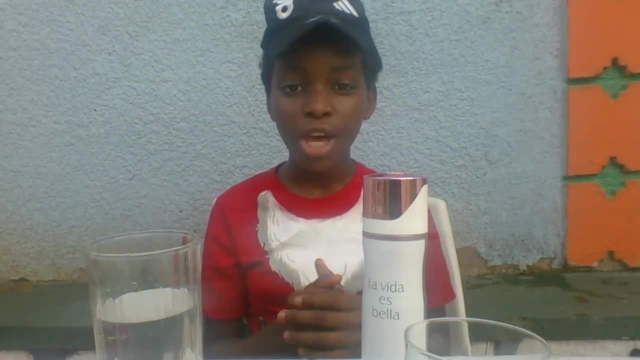 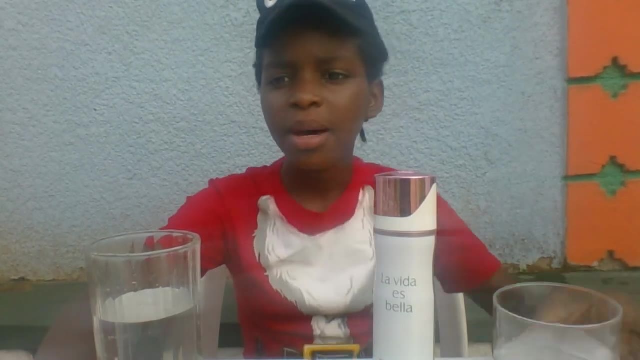 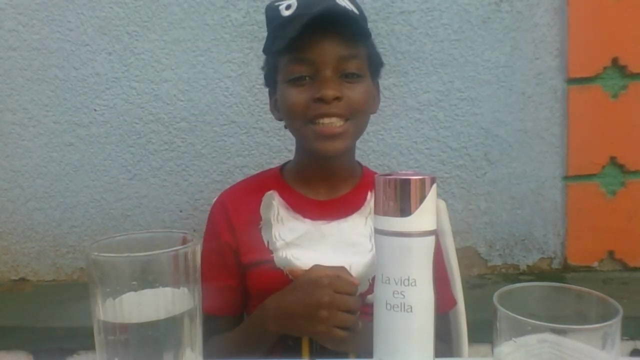 i guess it's like something with can see, yeah. so let's first: this is a solid, this is a liquid. we can see liquids, you can see solid, but the real question is: can we actually really see gases? sorry, the answer is no, we cannot see gases. but then what is the guys? so our guys also take the shape of its container, you see. 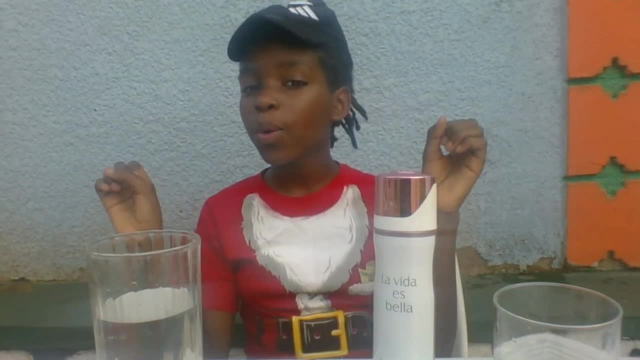 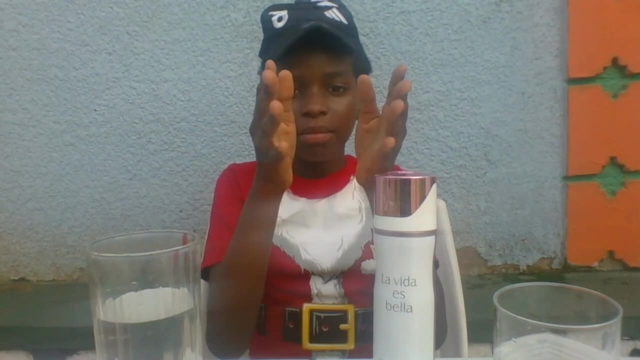 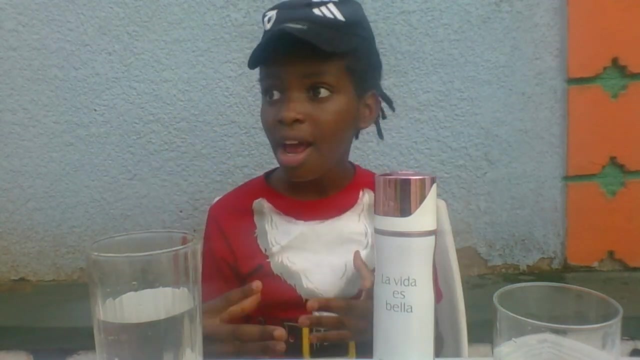 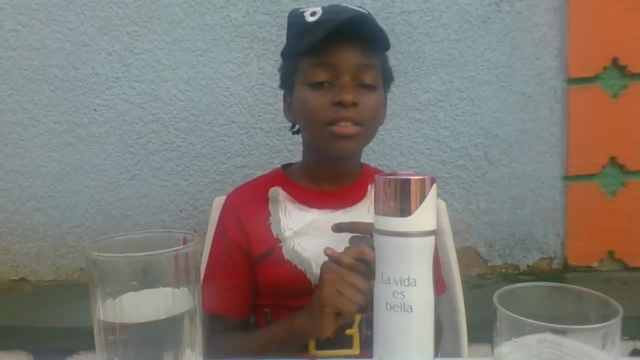 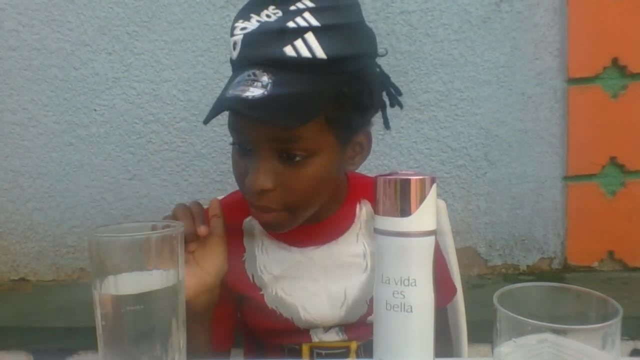 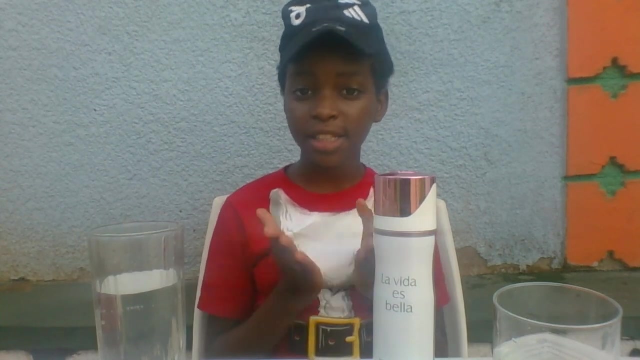 it. it's actually invisible, right? yeah, so you take this: the uh shape of each container, same as a liquid, but the only difference is that liquid we can see water, but actually gas can see. right, a gas can also change size and distribution. the gas can also take a particular shape of a container. 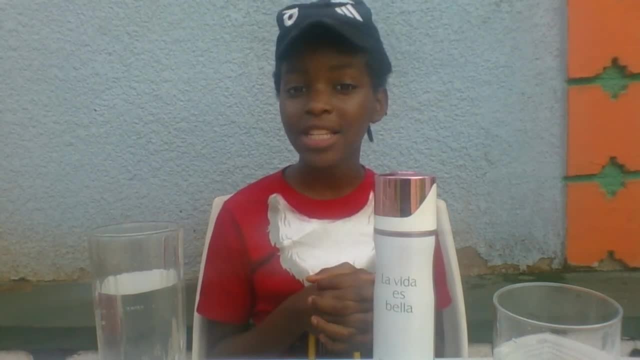 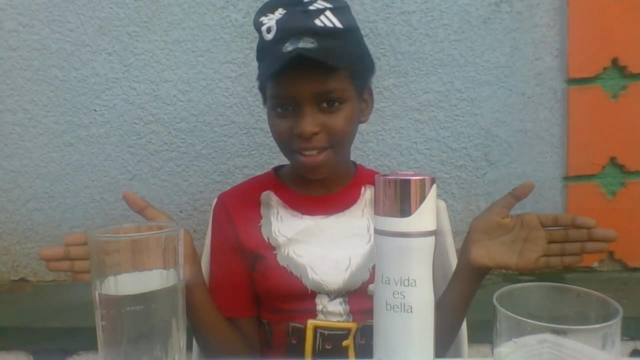 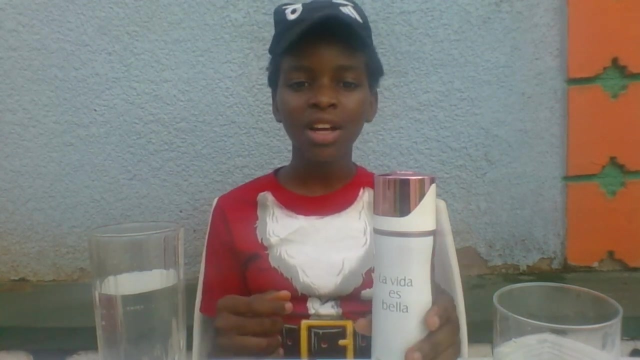 shape. i guess also fill up each container. it fills up like its container was like this. now it became like this. it is guys just fell in there. so this lesson actually was really easy and let's get some experiment. we're gonna see if this is actually a solid, a liquid or like us. 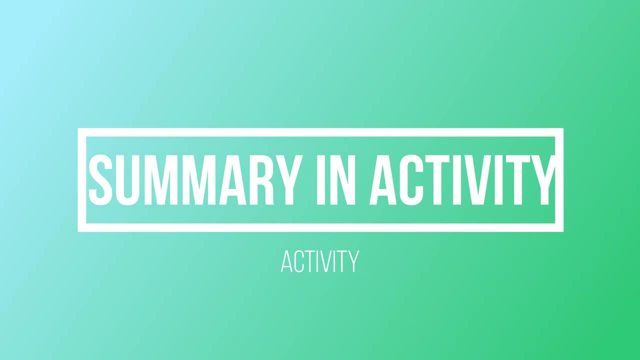 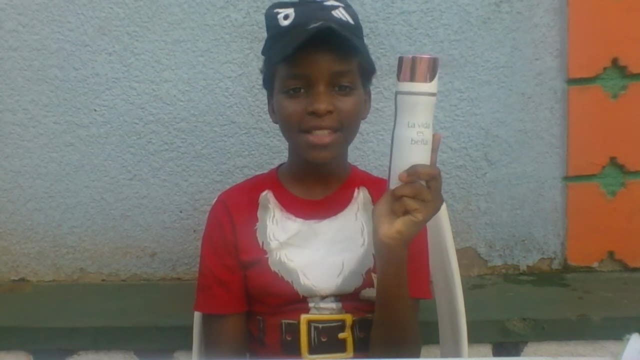 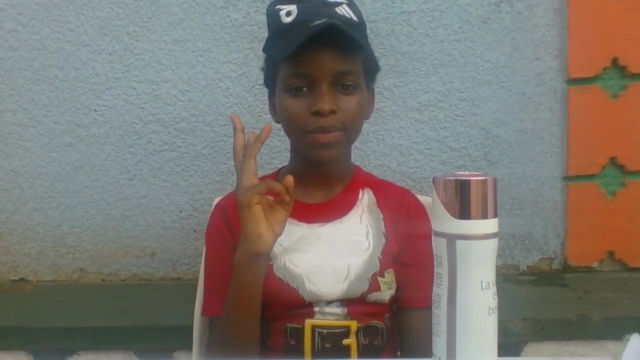 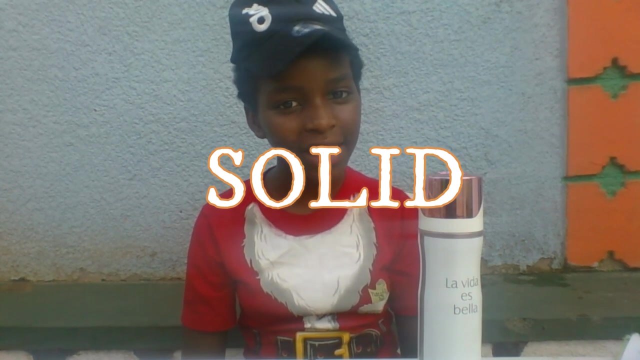 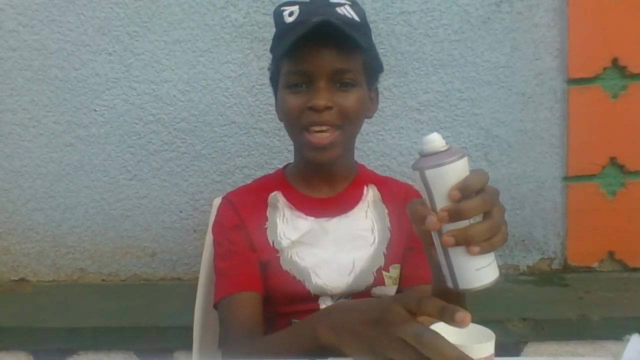 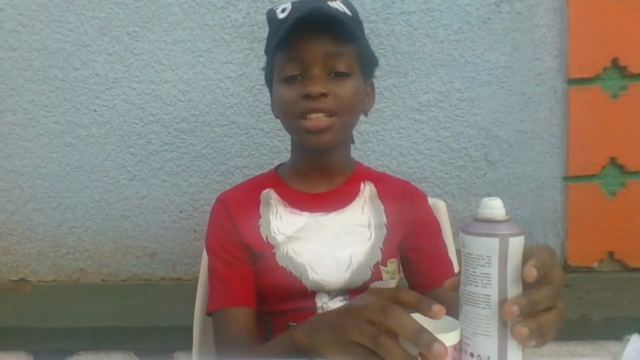 okay, guys, is this a solid, a liquid or a gas? three seconds respond, great job. it is a solid, but do we actually really have facts? that is a solid, let's find out. a solid has its own shape, let's see. wait, great, it has its own shape. when you move it, it can actually change. 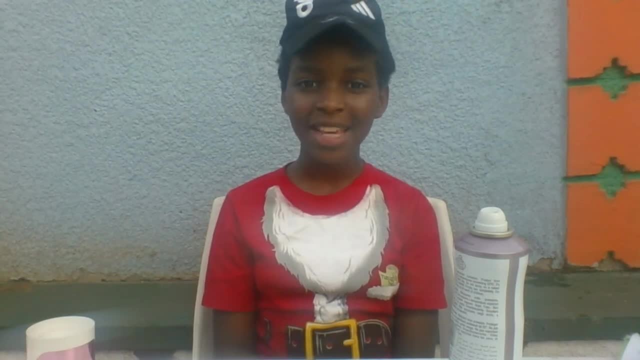 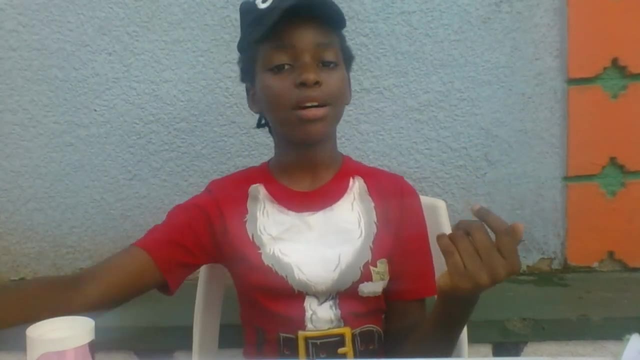 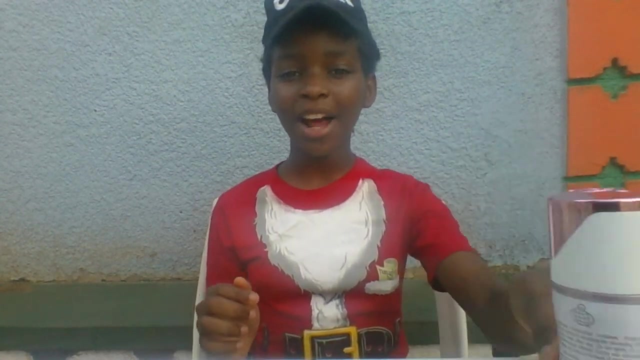 no, it can change. so it is a solid, yes, and it also has its own weight. let me put on a bonus: wow, it has its own weight. okay, these, we have product. it is a solid. now the second area: we're gonna actually need this, or maybe we can also use this. 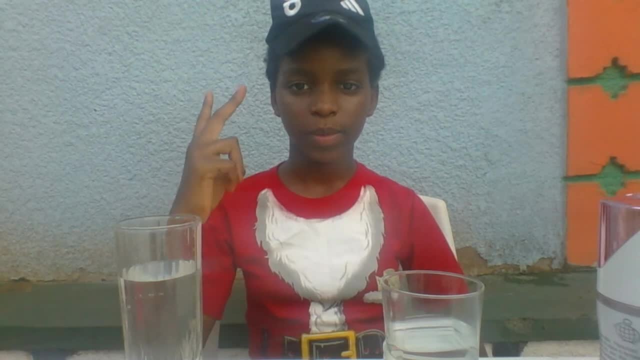 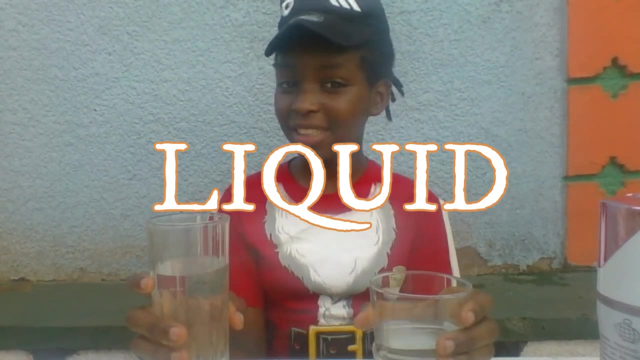 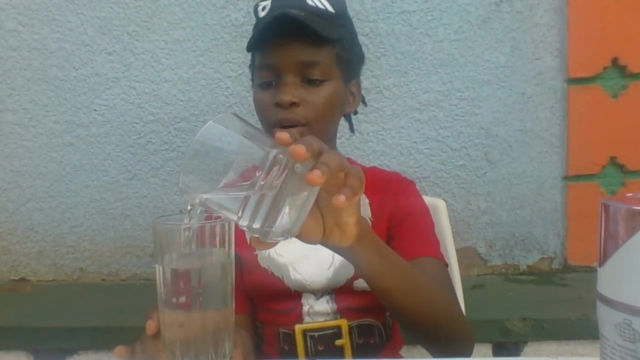 seconds to respond. this is a liquid. do you have facts? let's see, about its property? we see our liquids have shape of each container. let's see. let me first put all this water in here and then let's see if it can really have shape of its container. 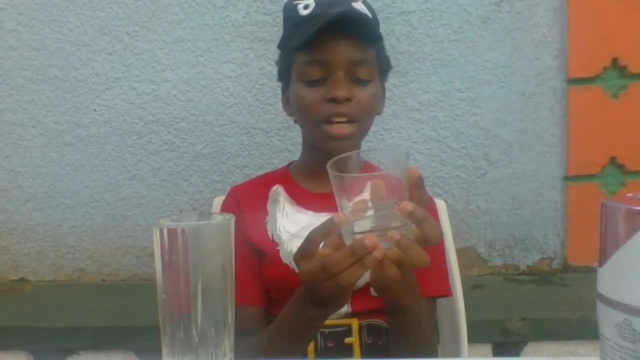 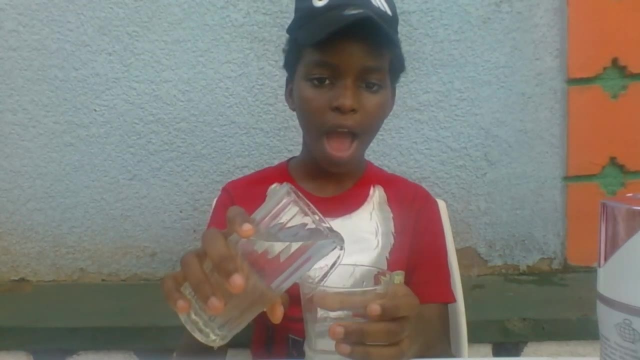 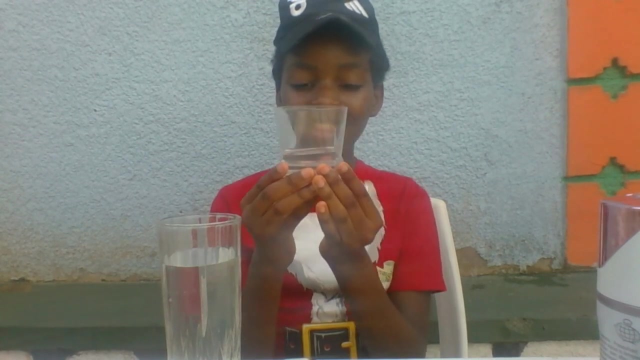 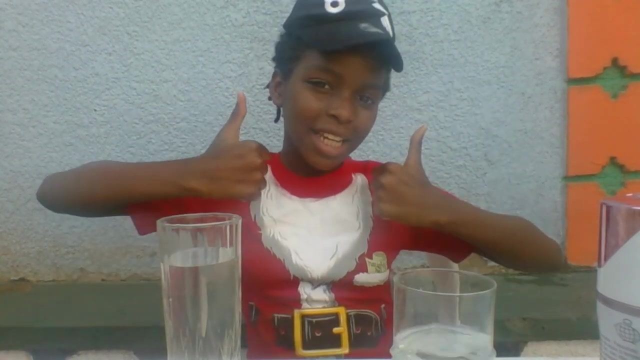 this is a container. this is another container. this one is actually different from this. let's see if you can also get sold out. yay, it can. it is a liquid. look at it's taking the shape of container, it's a little bit zigzag, and so on. it is. 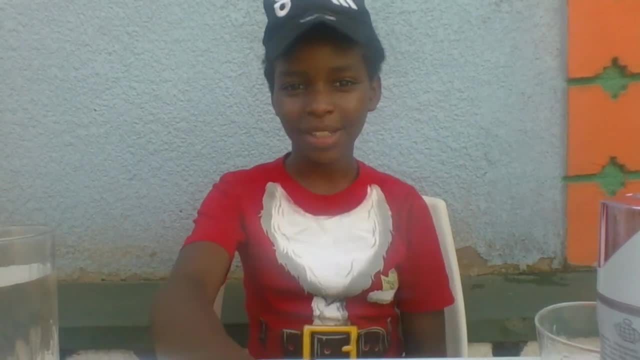 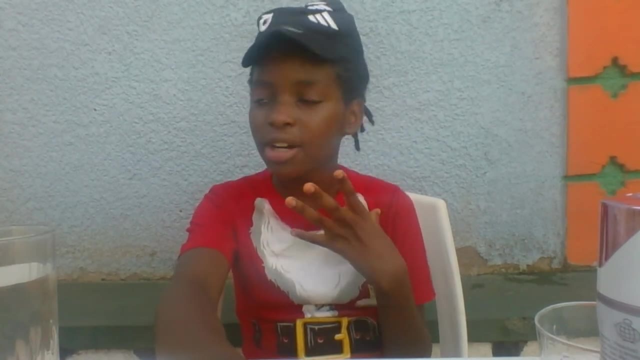 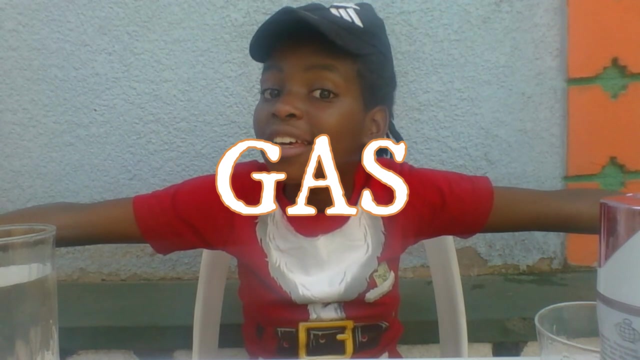 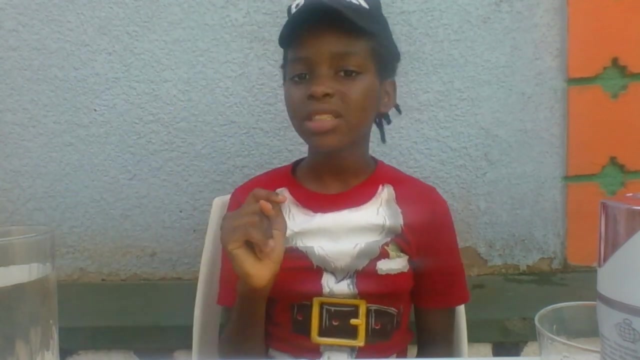 a liquid. now let's go to another object that you can see. this is a liquid or this is a gas, but actually a gas. when it's have a balloon, but actually I don't have a, you know, a gas, even this air is smelling. this air is smelling. it's a gas, why we can see, we can touch it, we can feel it, but 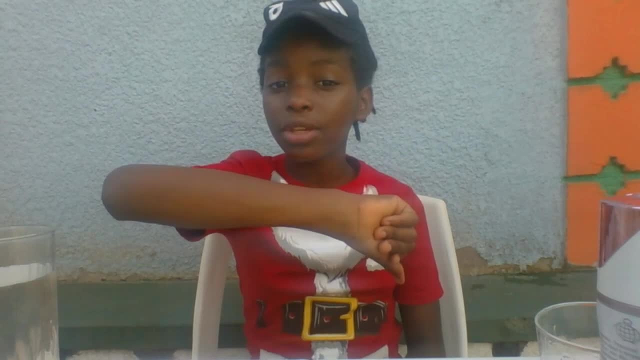 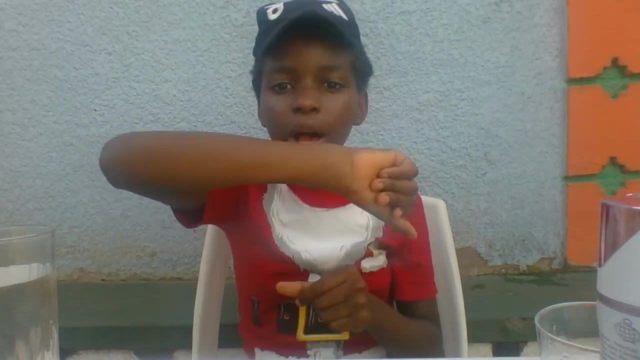 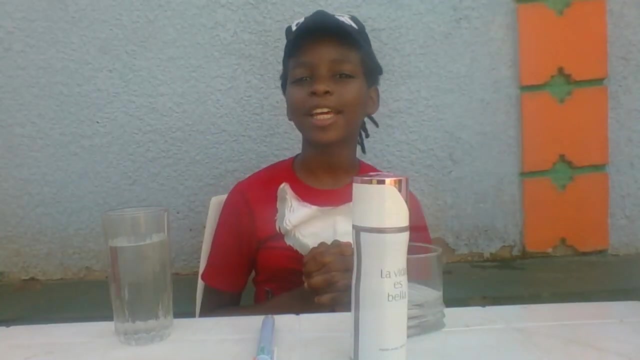 sometimes you can feel. what do you do that you can feel? can you see? can you touch it? you can only feel it. so, guys, that are all I have for you in this video and, as usual, don't forget to leave a very big thumbs up. subscribe to my. 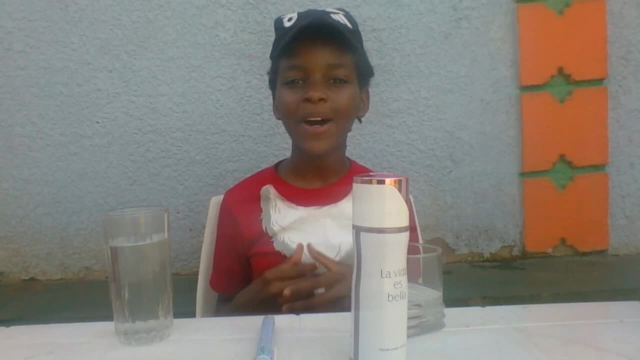 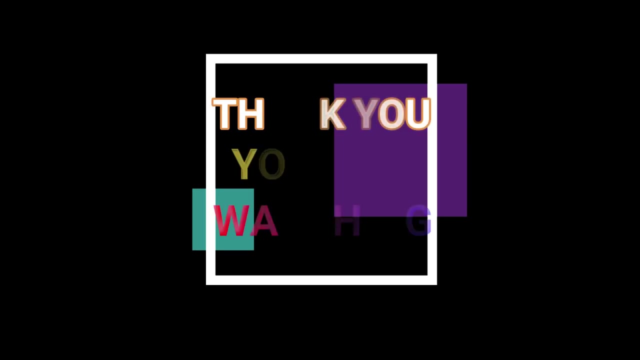